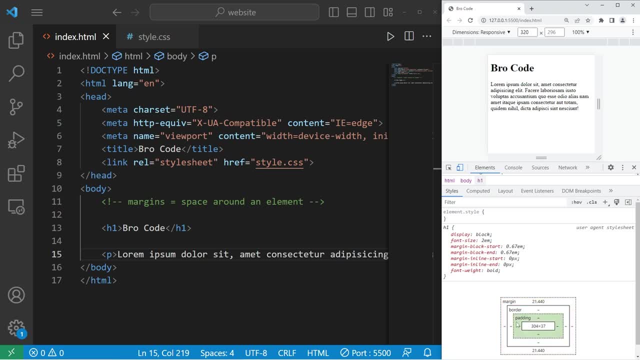 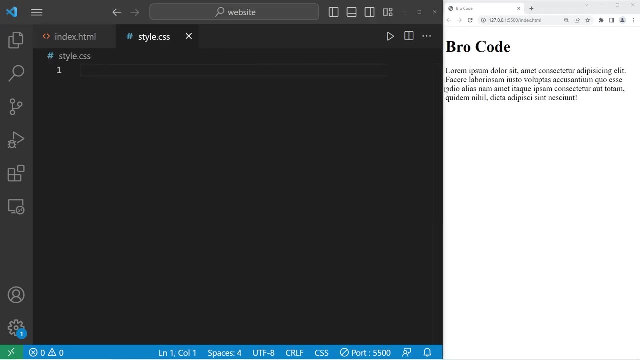 padding. border, then margins. Padding is between the element itself and any borders. Margins are the area outside of any borders. Today we'll be working with margins- the area outside of any elements. Let's close this window. Naturally, there's a few pixels of. 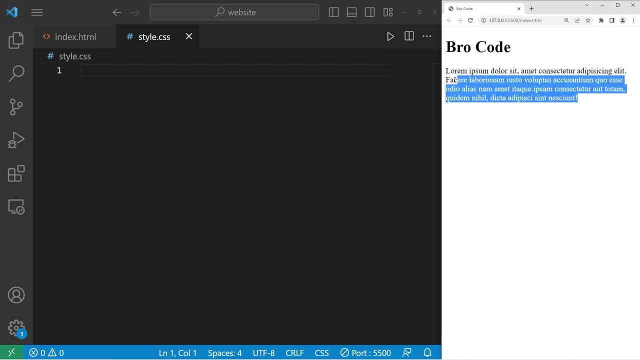 margin around our body and the letters in our H1 element and our paragraph aren't directly next to our pictures, which kind of looks like an onion. So to note that we need to get rid of the Rose's details so that our hydrogen is some improved perspective. 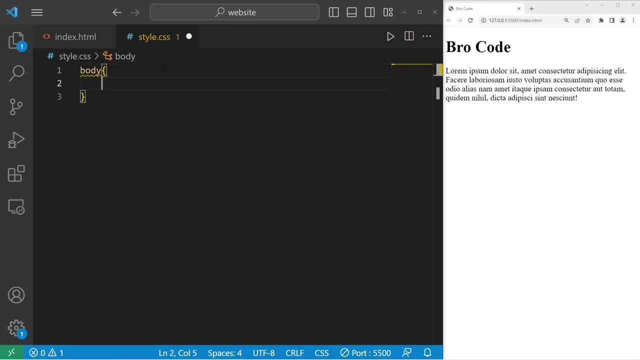 Some of our highlights are different, which are different from an IH Radiology photo. I hope that'll get better of our window So we can eliminate that. We will select the body element within our CSS style sheet. We will set the margin to be 0 pixels. So now the letters. 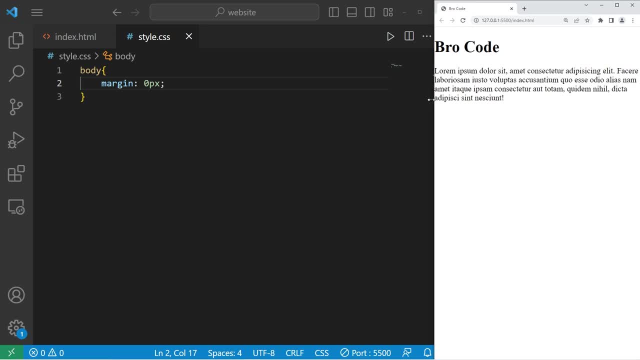 are directly next to the edge of the web browser And if I were to expand this, you can kind of see that. So that's all that margin is. It's the area outside of an element. To give you another example, let's delete our h1 element along with. 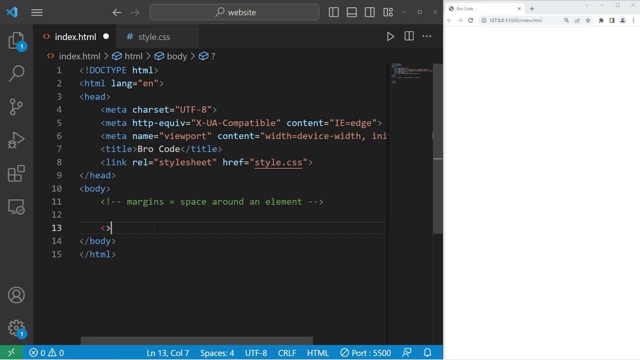 our paragraph. We'll create two div boxes. We need two pairs of div elements. I'll create a class for each of these divs class box. Then they will each have a unique ID. ID equals box1.. The ID for the second box will be box2.. And then 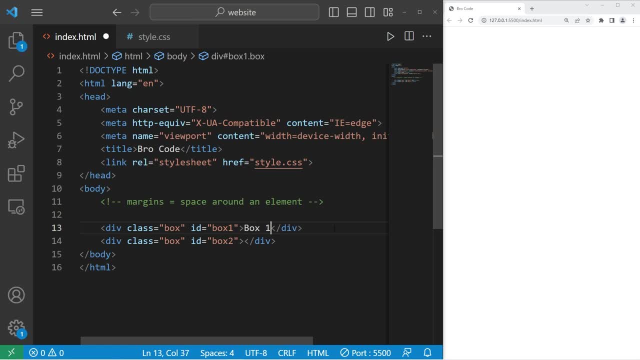 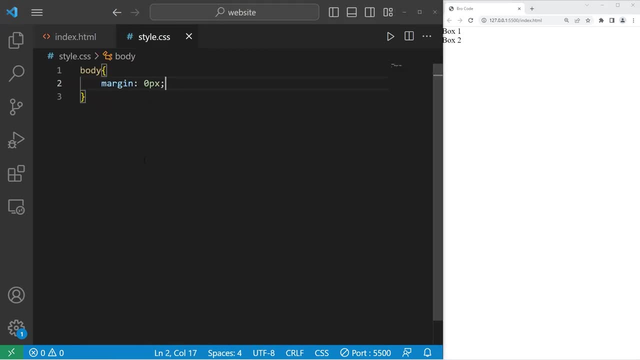 I'll give each of these some text: box1,, box2.. All right, Now let's style these boxes. So, after our body element, let's select the box class: Anything that's a box. let's add a border 5. 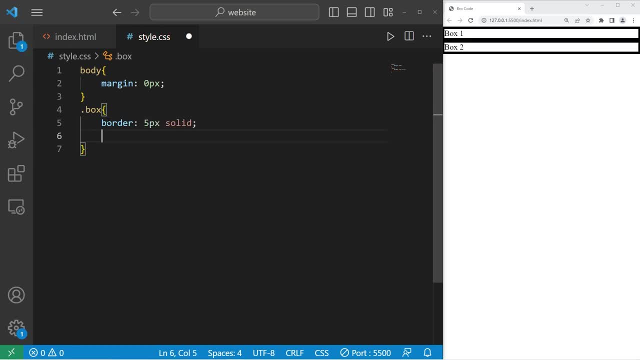 pixels. solid is fine. I'll change the font size to be 5em. Width, 250 pixels, Height, 250 pixels, And I'm just gonna zoom out a little bit until our view is at 100%. Let me color box1 and box2.. We are selecting the ID of box1 for. 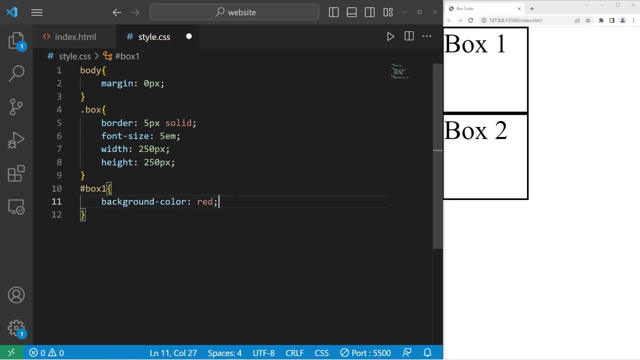 the background color. Let's set that to be red, But let's select a more custom red because it's cool. All right, Then box2 will be blue. All right, There are marginal directions. We can apply margin to the top of an element, the right, the bottom or the left. 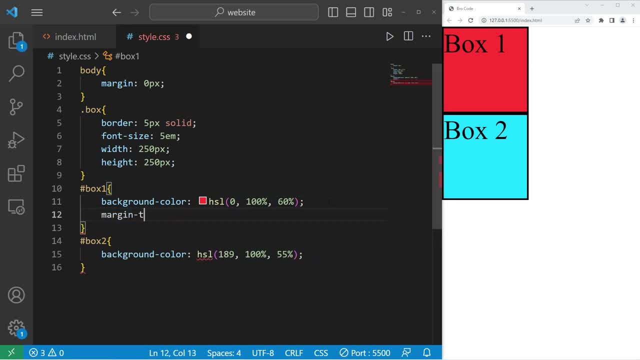 or all sides With box1. I will set a margin-top property to be 50 pixels. That's going to add 50 pixels of margin at the top of this element, box1.. There's also margin-bottom. Now there's 50 pixels of margin at the bottom And then, as you can see, you can assign all these objects to this div. 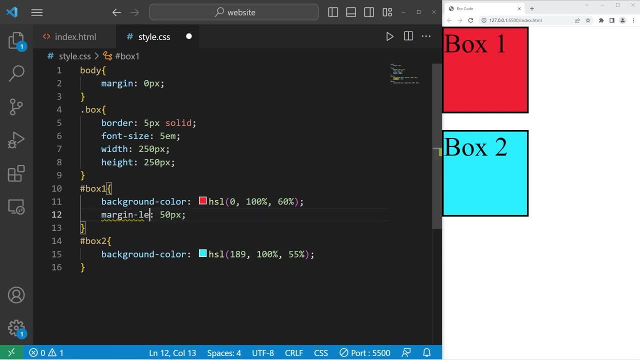 of margin after box one: Margin left: The margin is now on the left. Margin right: The margin is now on the right. but you can't see that because divs are block level elements. They take up the entire horizontal space. You could apply margin to all sides evenly, just with margin, So margin. 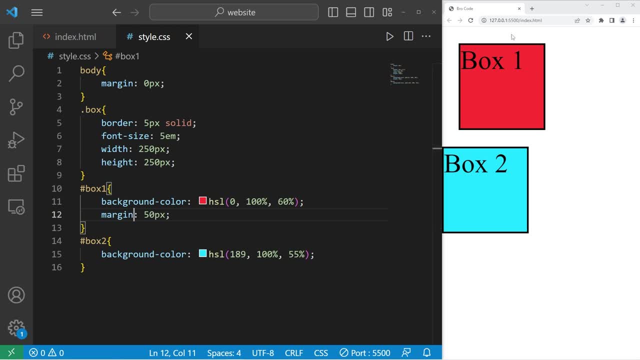 50 pixels. That applies 50 pixels of margin to the top right, bottom, left. So if we were to apply this margin to a class like the box class, both box one and box two will have 50 pixels of margin around each element. There's also margin auto. It is possible to set an element's margin. 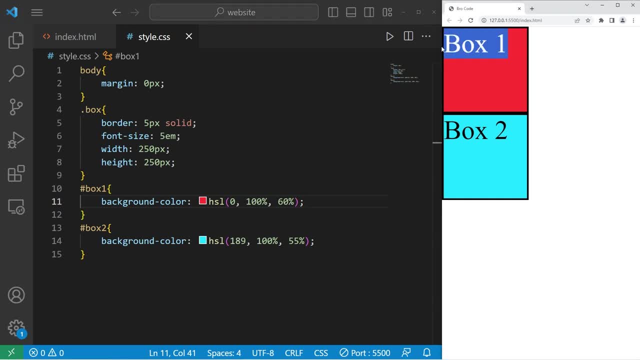 to take up the entire space. I can take any of these elements, such as box one, and push it all the way to the right of my web browser using margin left, Margin dash left. Then I will set it to be auto. The margin auto is set to the right of my web browser using margin left, Margin dash. 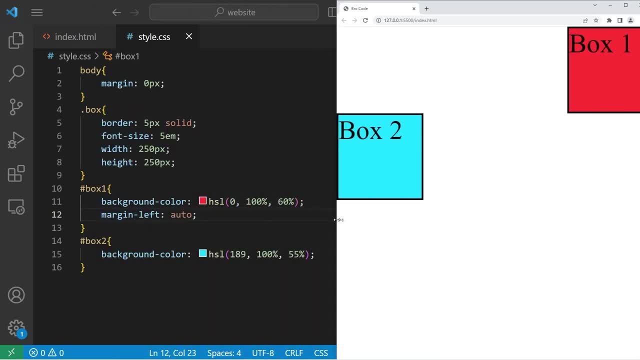 left, Then I will set it to be auto. The margin auto is set to the right of my web browser using margin right. The margin auto is set to the right of my web browser using margin left. So the margin on the left side of box one will take up as much room as possible. So box one is going to stick. 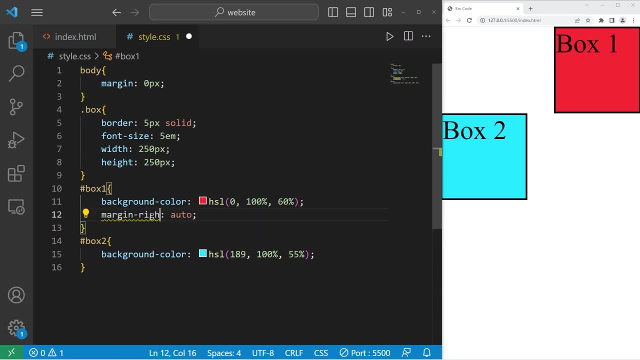 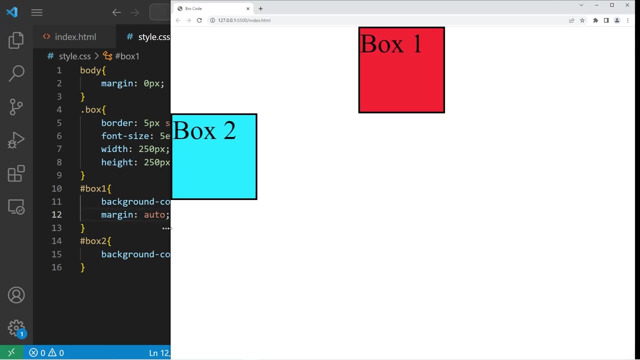 to the right hand side of the web browser. Margin right won't appear to do anything because it's already left justified. Now, if you would like an element to stay in the center of your web browser, you can just set margin to be auto, So box one is going to stay in the middle.